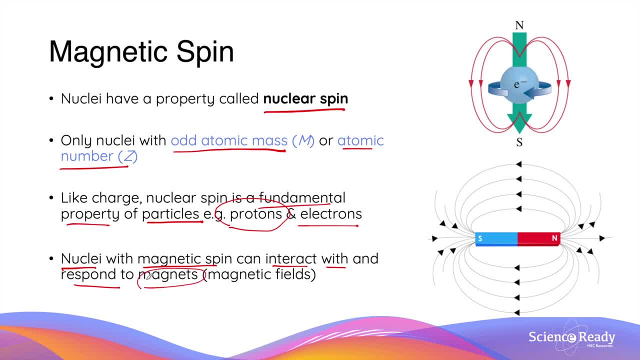 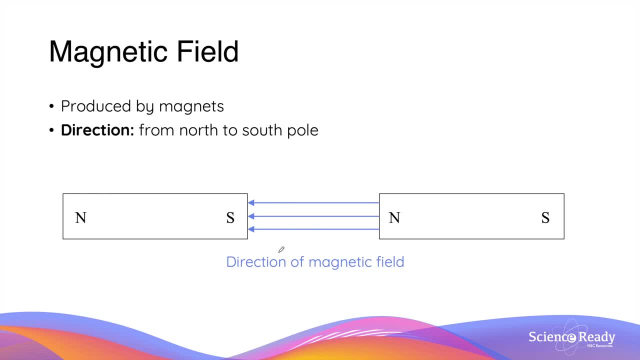 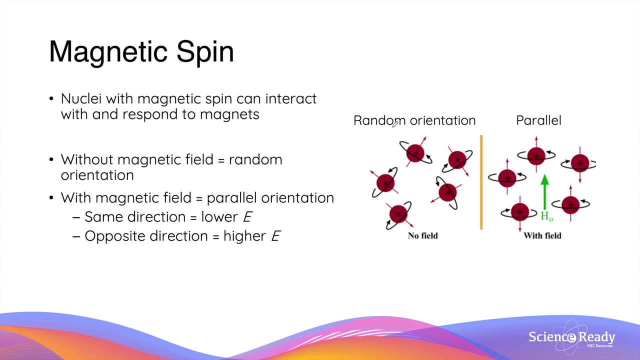 interact with and respond to the magnetic spin of nuclear particles. A pair of magnets can be used to produce an external magnetic field, where the direction of the magnetic field goes from the north pole of one magnet to the south pole of the other. In the absence of a magnetic field, the nuclear spin are randomly orientated. 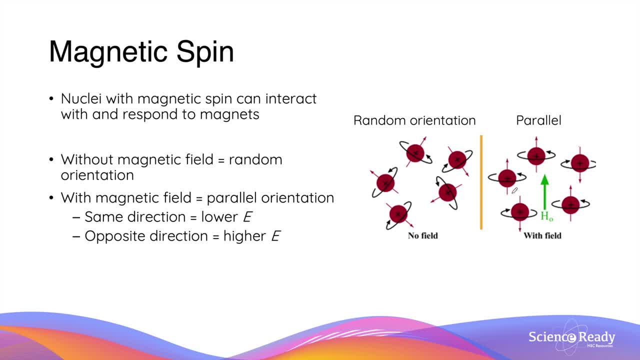 However, upon applying an external magnetic field, the spin of nuclei become parallel to the field. When they are parallel, some nuclear spins can be in the same direction as the magnetic field, while the other ones will pose the field. It's important to keep in mind that the direction of these spins determine the 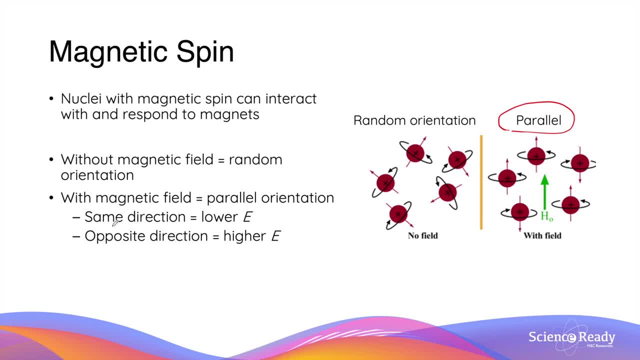 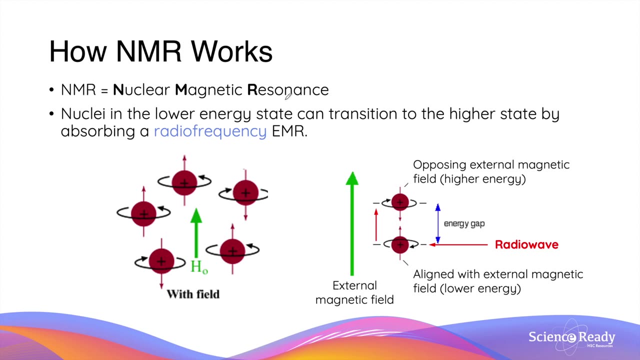 energy level of each nucleus, such that nuclei which are pointing in the same direction as the magnetic field have a lower energy and those which are posing the magnetic field have a higher energy. MMR, which stands for nuclear magnetic resonance, uses radio waves. 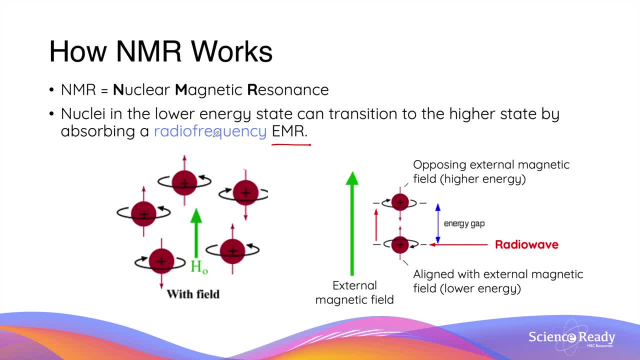 a type of EMR to interact with nuclear spins which are subject to an external magnetic field. Specifically, nuclei which are in the lower energy state can transition to a higher state by absorbing a specific frequency of radio waves In terms of their orientation. when a radio wave is blasted at a nucleus upon absorption, 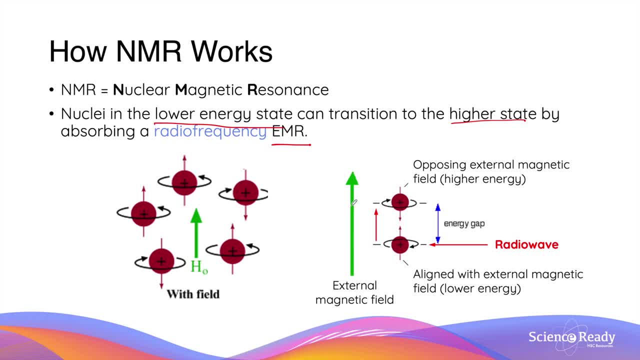 a nucleus which is originally pointing in the same direction as an external magnetic field can tip its direction such that it adopts a direction that is opposite to the field. This means nucleus which was originally in a lower energy state can reach a higher energy state. The phrase nuclear magnetic resonance refers to when a particular nuclear spin responds. 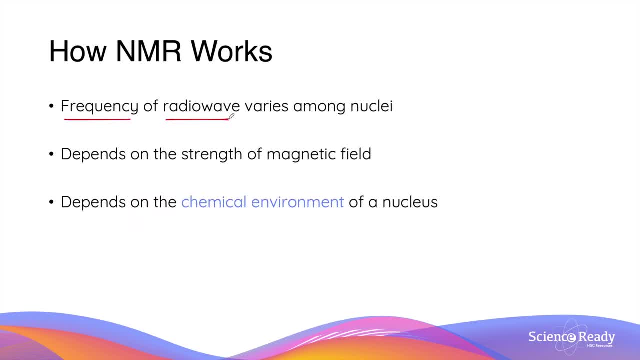 to the radio wave. Frequency of radio wave that is absorbed by the nuclei varies among different nucleus. This depends on two factors: The frequency depends on the strength of the external magnetic field that is being used and also, more importantly, the chemical environment of a particular nucleus. 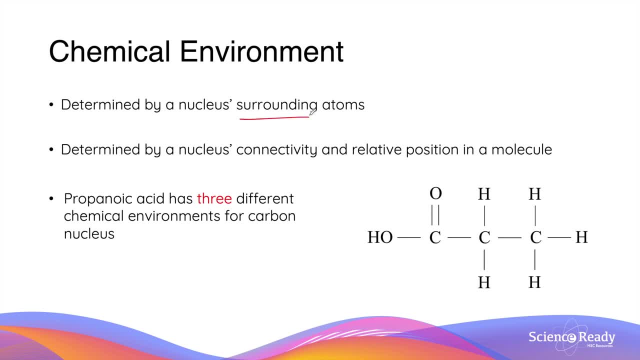 The chemical environment is determined by a nucleus surrounding atoms, as well as connectivity and also the relative position of the atom in the molecule. For example, if we are examining the molecular structure of propanoic acid, there are exactly three chemical environments for the carbon, because each carbon atom is connected to. 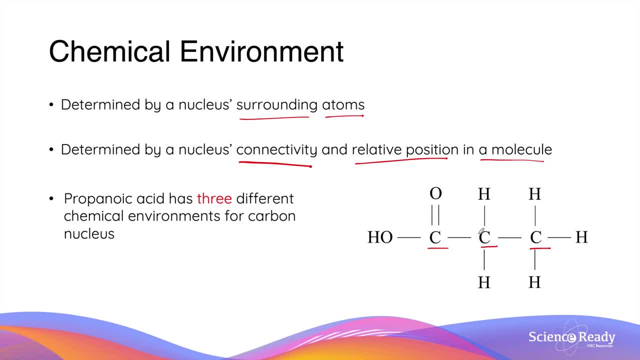 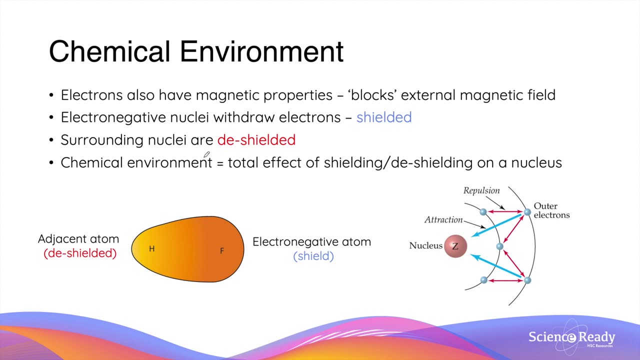 surrounding atoms differently compared to the other two. At the same time, each carbon's relative position in the molecule compared to the other atoms is also slightly different. The reason why connectivity and relative position of a nucleus affects its chemical environment and the frequency of radio wave that it can absorb at is because electrons which surround 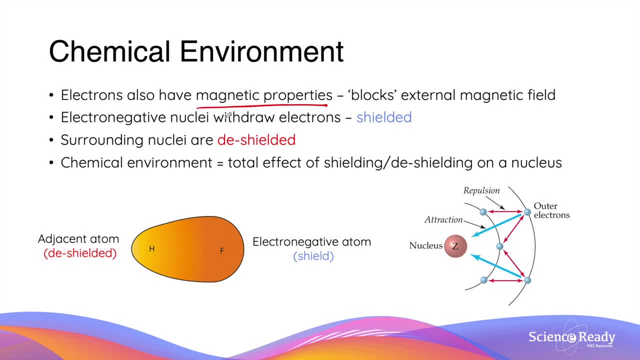 the nucleus also have magnetic properties, and the magnetic properties of the electrons have the ability to block the external magnetic field that is subject to the nucleus. Electronegative atoms or nuclei have the tendency to withdraw or attract electrons that surround them. This gives them a shielding effect, which means they are less affected by the external magnetic. 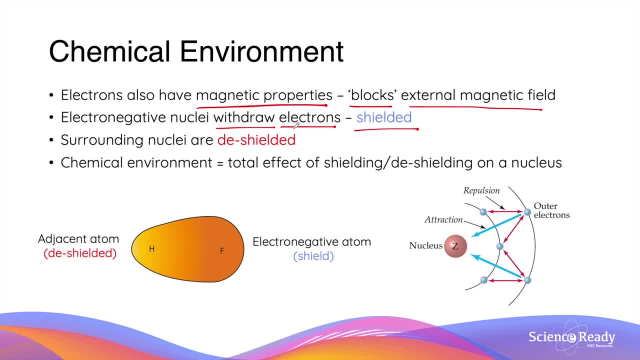 field. When the electrons are being drawn or attracted away from the nearby atom, they become shielded by these electron-negative nuclei. The surrounding nuclei are described as deshielded. that is, the effect of the external magnetic field becomes greater for the surrounding nuclei. Let's look at a simple example. If we have a hydrogen atom adjacent, 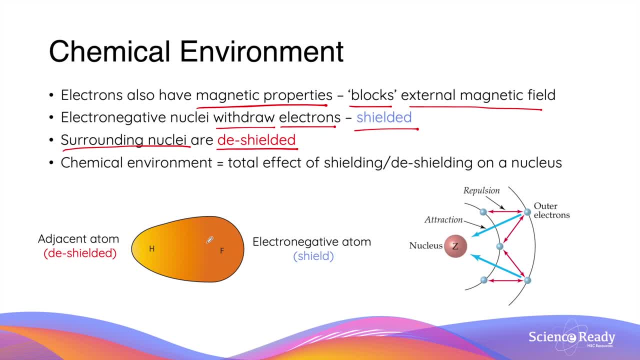 to a very electronegative atom such as fluorine. the fluorine will withdraw its surrounding electrons so that it becomes shielded, while the hydrogen atom, whose electrons are being drawn away from it, will be shielded. This is because the electrons are being drawn away. 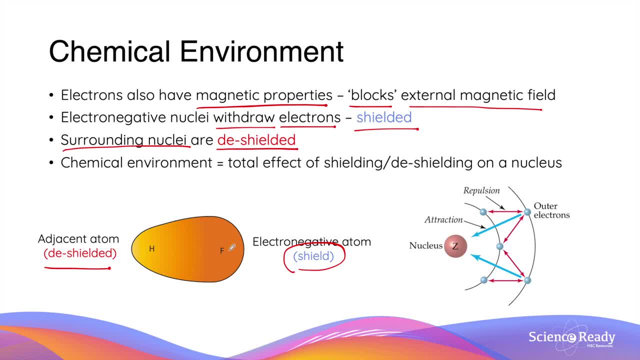 from it and the electrons are being drawn away from it and the electrons are being drawn away from it. In other words, the fluorine atom becomes less affected by the external magnetic field, while the hydrogen atom becomes more affected. The term chemical. 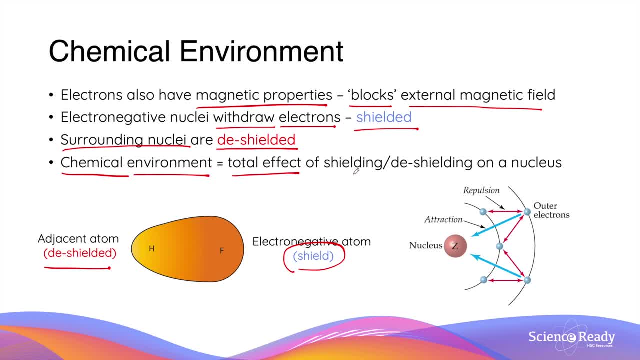 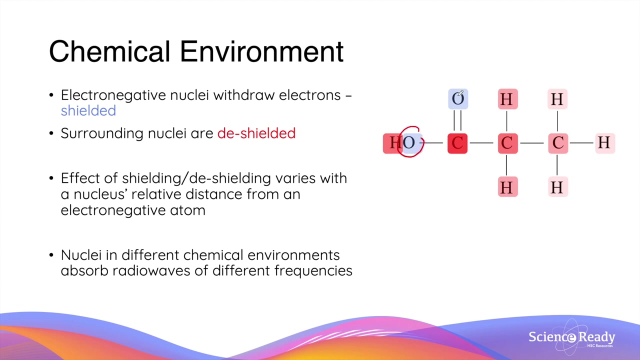 environment therefore refers to the total effect of shielding or deshielding of a nucleus. This is why the chemical environment is affected by the adjacent atoms as well as the relative position of the nucleus within the molecule. Let's apply that example to propionic acid. In propionic acid, there are two oxygen atoms. 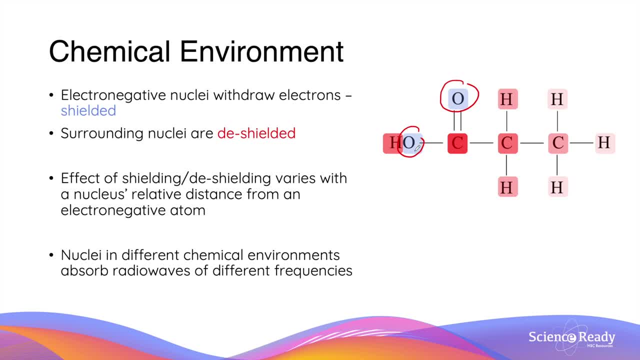 which are both electronegative. Therefore, they will attract electrons surrounding them, causing atoms nearby to become deshielded, Depending on the relative distance of the atom or nucleus from these two oxygen atoms, the extent to which they are deshielded by.